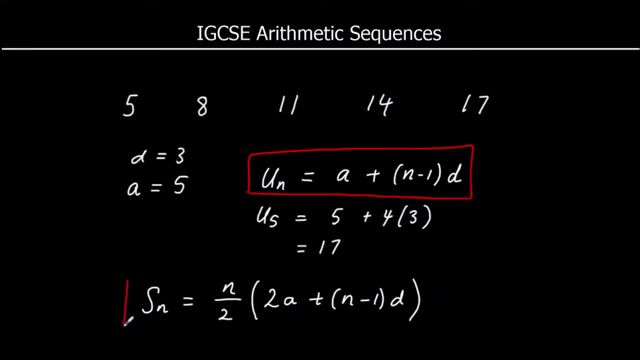 So we can use this formula to find the sum of some terms in the sequence. So if we wanted the sum of the first five terms, if we want to add all these up, we could substitute in n as 5, a as 5, and d as 3, and it will tell us what these first five terms add up to. 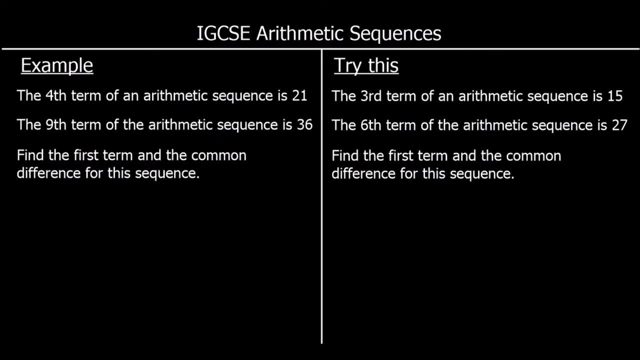 Let's have a look at some questions. So this example says the 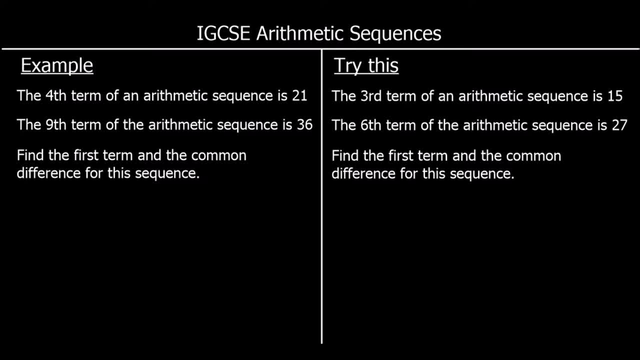 fourth term of an arithmetic sequence is 21. The ninth term of the sequence is 36. Find the first term and the common difference. So we're not looking at the sum in this one. 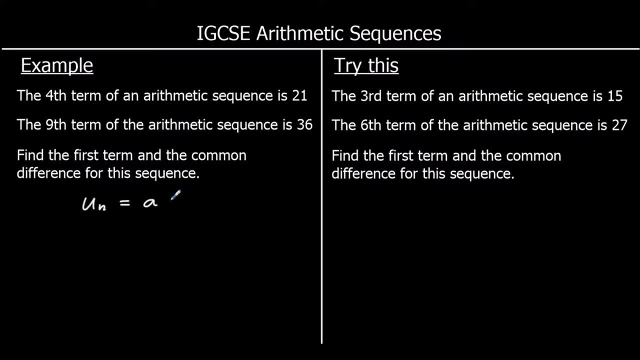 So we're going to be using un is a plus n minus 1 times d. So we know the fourth term, so u4 is 21. So we can write 21 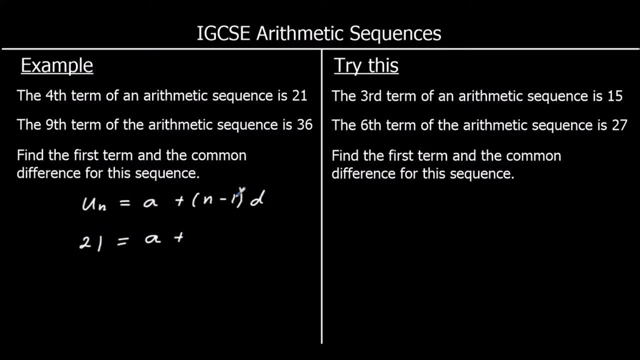 is a plus four minus one so 3, lots of the common difference. 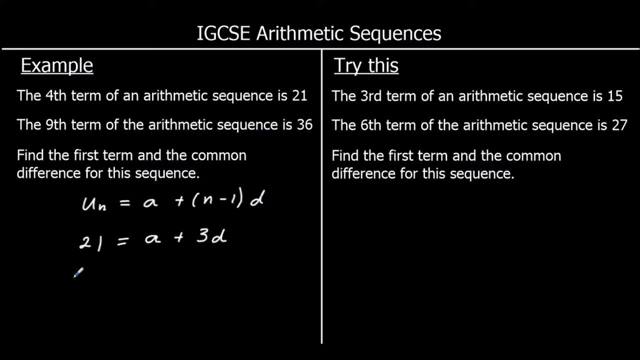 The ninth term is 36. So 36 is a, plus 9 minus 1, 8, lots of the common difference. 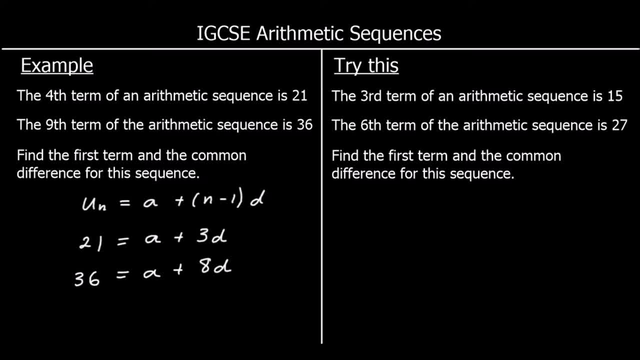 We've got simultaneous equations now. We can solve them by taking away We've got A in both. So if we take away the top equation from the bottom equation, we're going to eliminate A. 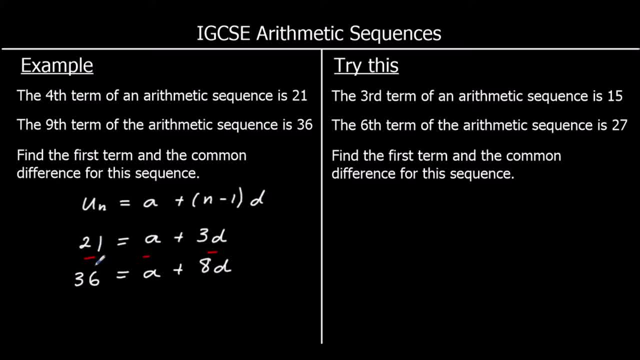 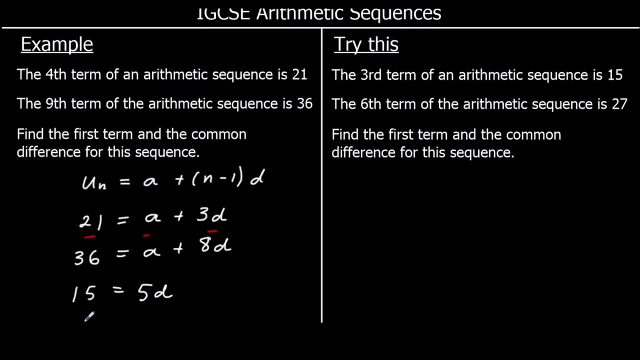 So 36 take away 21 is 15. A take away A is nothing. And 8 Ds take away 3 Ds is 5 Ds. So 15 equals 5 D. Divide both sides by 5. 5 D equals 3. 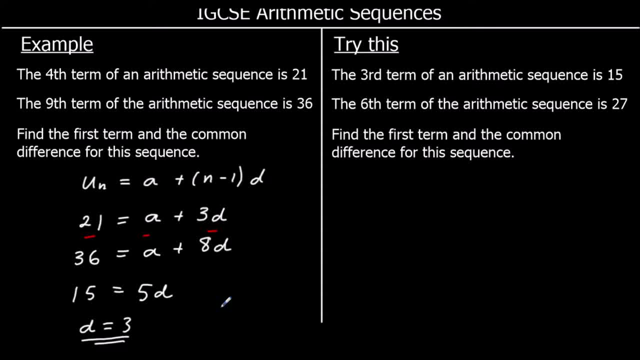 The common difference of this sequence is 3. 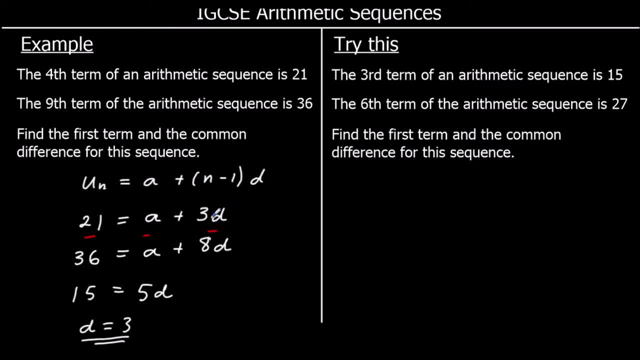 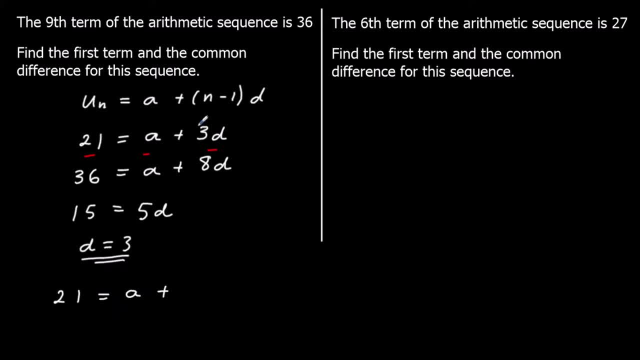 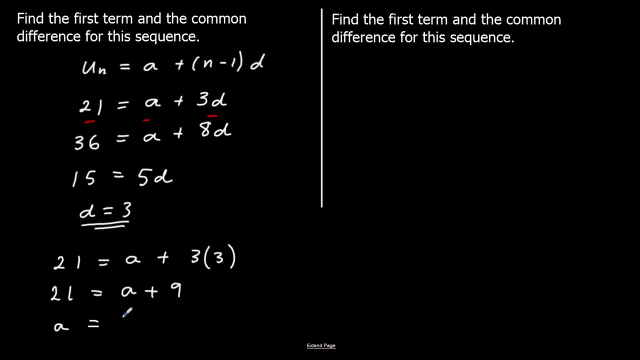 Now we can substitute that back in to one of our equations and find A. So we can say 21 is equal to A plus 3 Ds. D is now 3. 3 3s. Which are 9. So 21 equals A plus 9. Take 9 away from. Both sides. A must be 12. 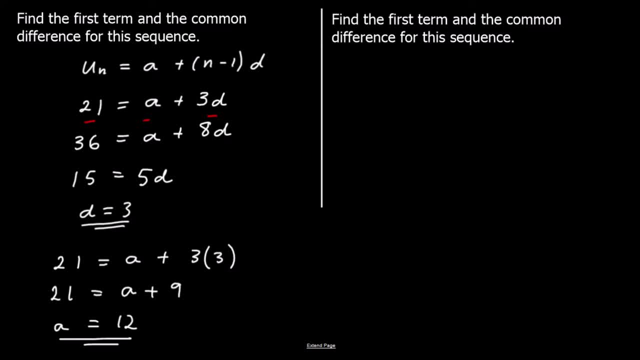 So there we've worked out our first term and our common difference. So here's one for you to try. Pause the video and give it a go. 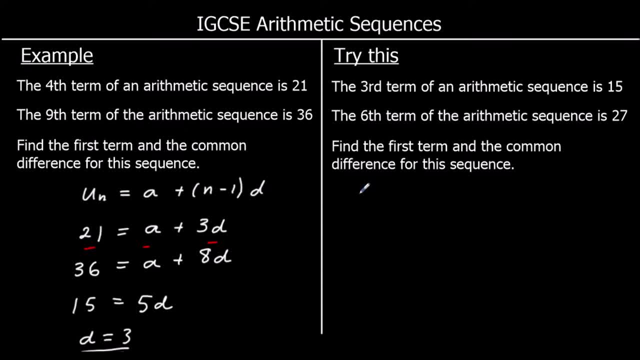 So again, we're using the same formula. un equals A plus n minus 1 times D. We're told the third term is 15 and the sixth term is 27, and we need to find A and D again. So the third term is 15. So 15 is the first term plus 3 minus 1. So two lots of the common difference. 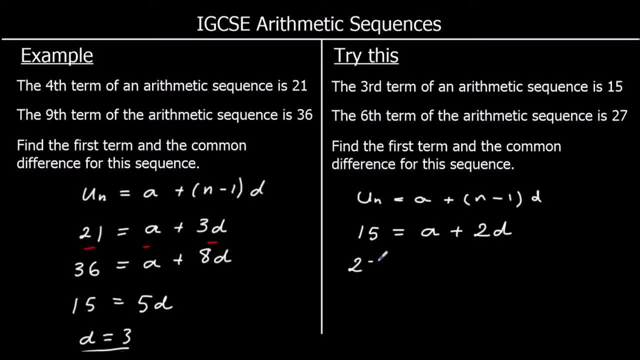 The sixth term is 27. So 27 is the first term plus n minus 1. Six minus 1 is 5. Five lots of the common difference. 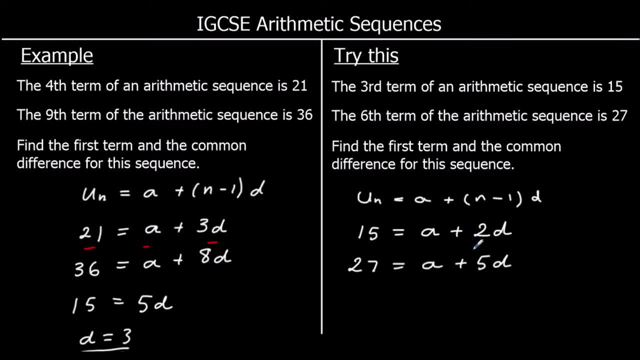 We need to solve these simultaneous equations now. We've got two equations, two unknowns that make some simultaneous equations. And if we solve them, we find A and D, which is what we want. So again, A is, we've only got one A in both equations. We can eliminate it by taking one equation away from the other. 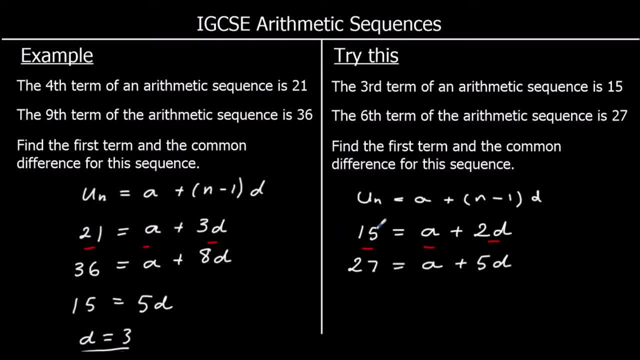 So I'm going to take the top one away from the bottom. 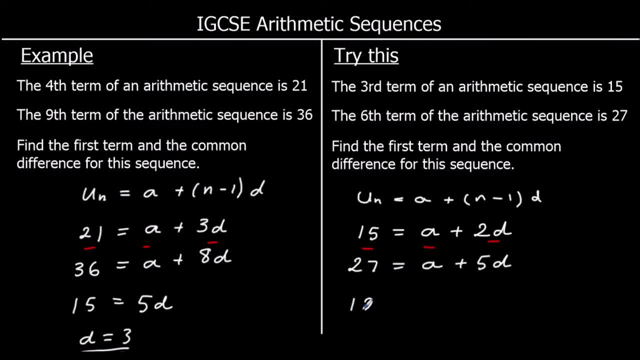 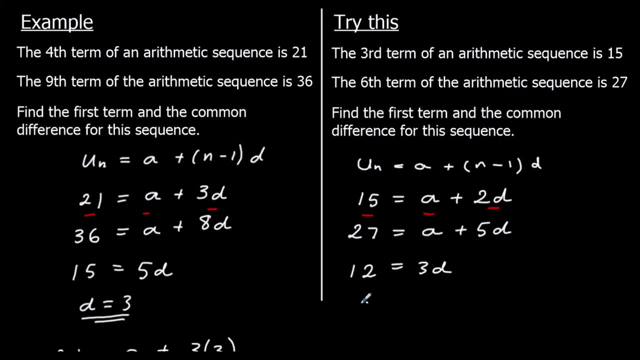 So 27 take away 15 is 12. A take away A is nothing. Five take away 2 is 3. So we've got three Ds. 12 equals 3D. Divide both sides by 3. And that gives us D is 4. Let's substitute this in to find A. 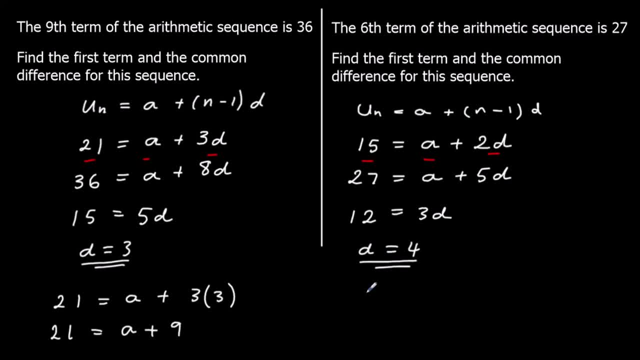 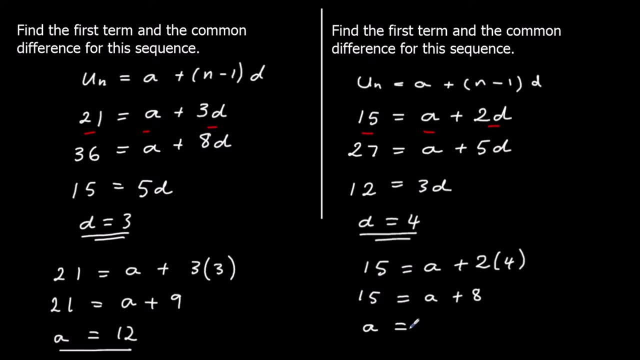 So let's go into the top equation. 15 equals A plus two lots of the common difference. So 15 is A plus 8. Take 8 away from both sides. And we get A as 7. 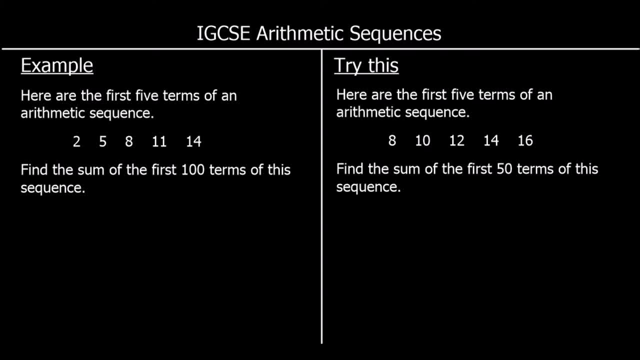 Here's another example. We've been given the first five terms of a sequence. 2, 5, 8. 8, 11, and 14. 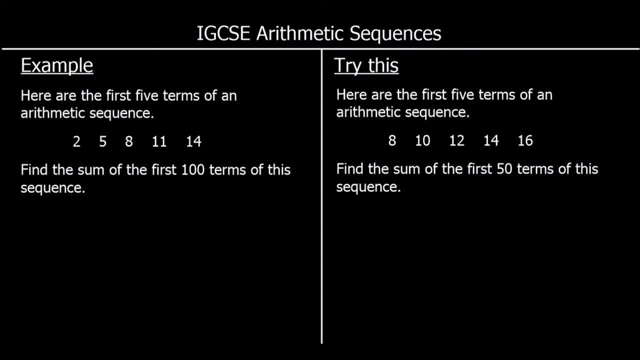 And we want the sum of the first 100 terms. So we're finding the sum. 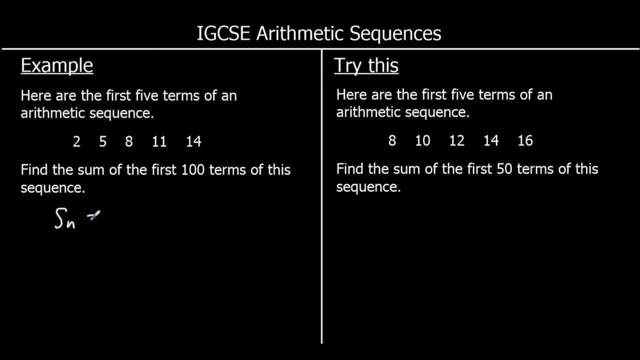 We're going to be using our sum formula, which is SN equals N over 2 times 2A plus N minus 1D. 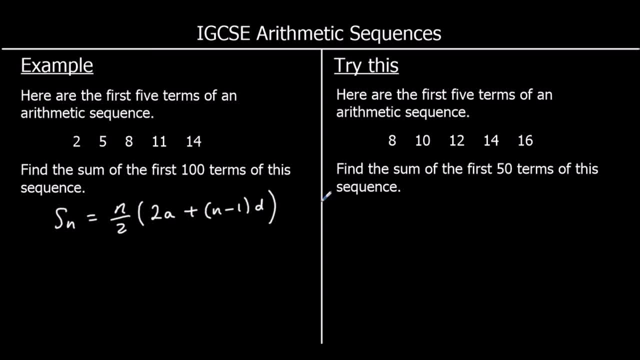 We can write down what A and D are this time. So N is 100. We want 100 terms. So N is 100. 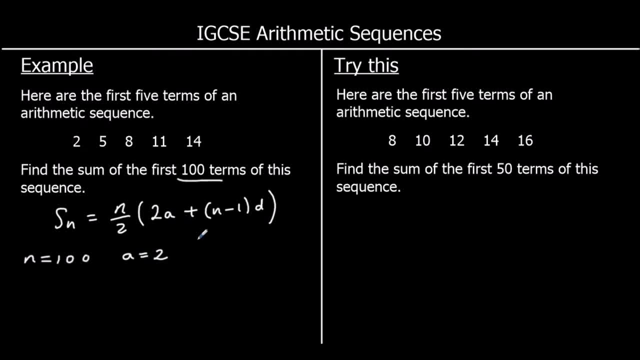 A is the first term, which is 2. And D is the common difference. It's going up in 3s. So D is 3. 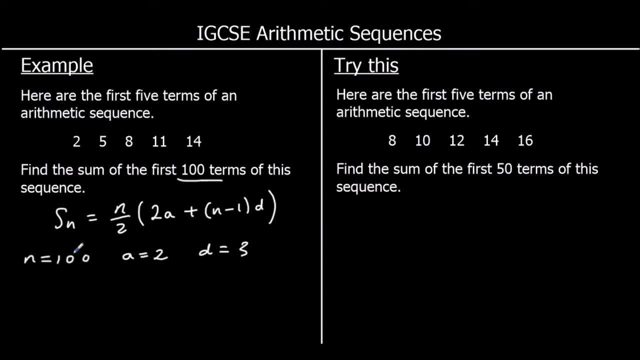 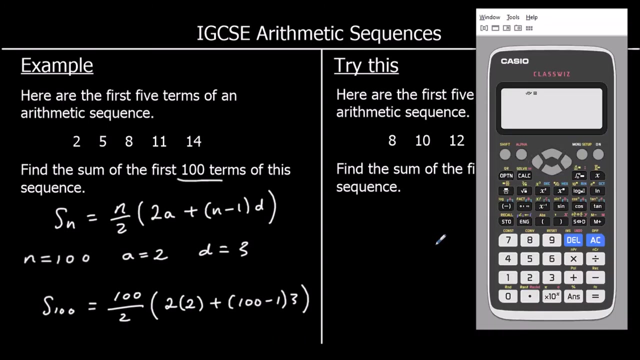 And we're just going to substitute these values in. So it's the sum of the first 100 terms will be equal to 100 over 2 times 2A, which is two 2s, plus N minus 1. So 100 minus 1 times the difference, which is 3. And we can type that into a calculator. So we'll grab a calculator and type it in. 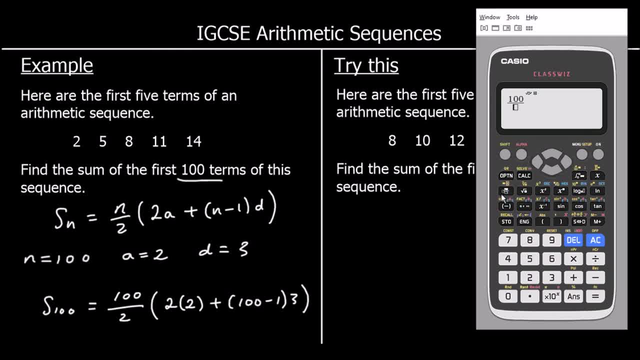 So we've got 100 over 2 times two 2s, 2A, plus N minus 1. 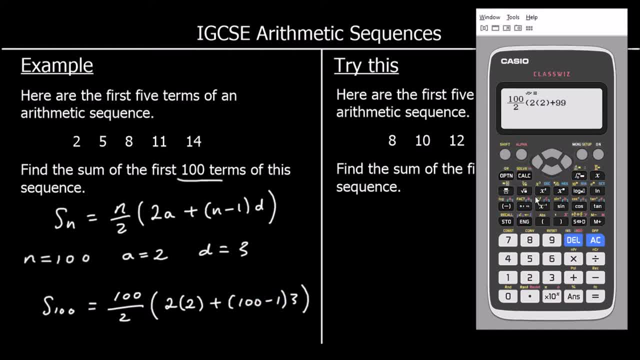 I'm just going to write as 99. 100 minus 1, I'm going to write as 99, times 3, and press equals. 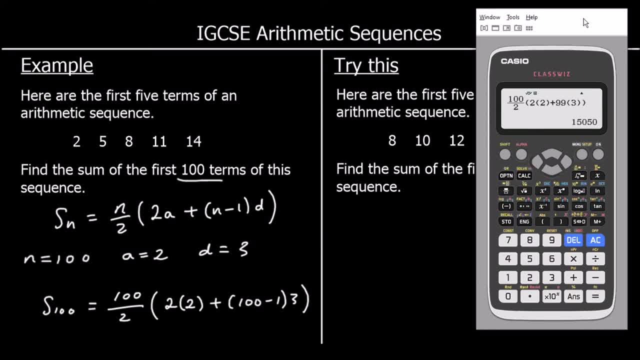 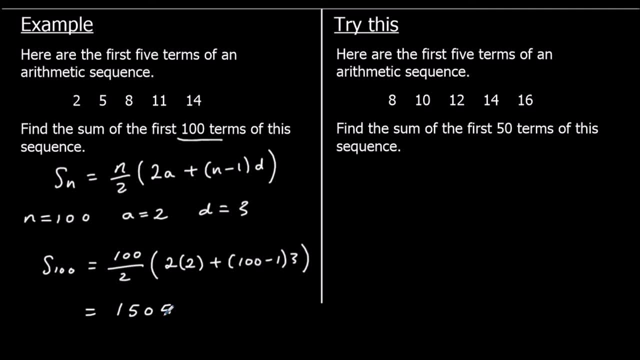 And there's our sum, say 15,050. So the sum of the first 100 terms is 15,050. So if we kept this sequence going for 100 terms and added them all together, this is what we'd get. So if we kept this sequence going for 100 terms and added them all together, this is what we'd get. 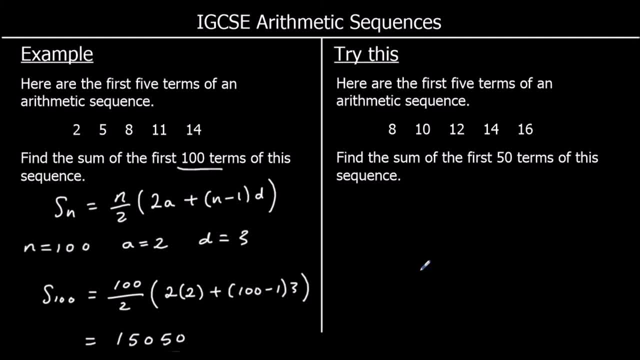 And here's a question for you to try. So pause the video and give this one a go. 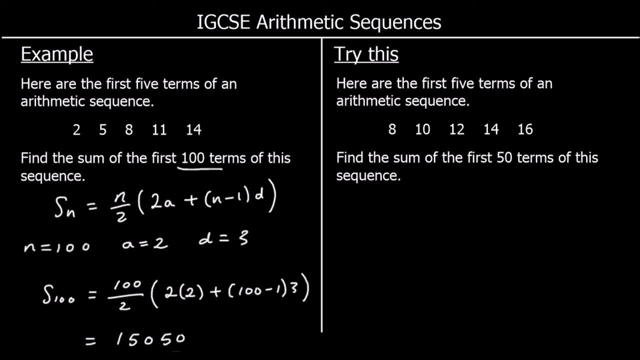 OK, so again, we've been given the first five terms. So and we need to add up 50 terms. So N is going to be 50. The first term of the sequence is 8. And this time the common difference is 2. It's going up in 2s. So we're substituting into the formula. So the sum of the first 50 terms. So the formula is written down here. 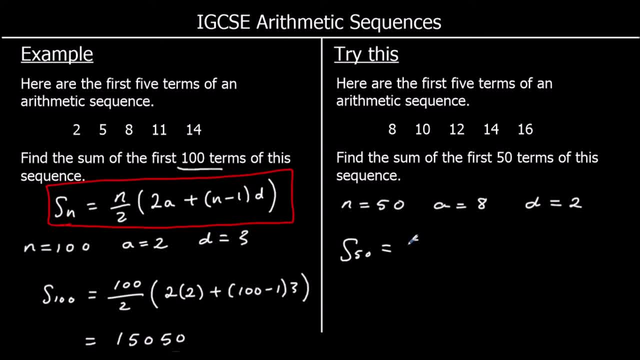 The sum of the first 50 terms is N over 2. So 50 over 2 times 2 eighths plus N minus 1. 50 minus 1 is 49 times the common difference, which is 2. And we can type it in the calculator. 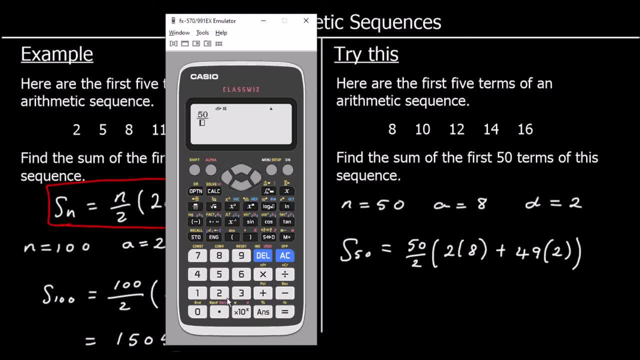 So we have 50 over 2 times 2 eighths plus 49 times 2. And that's 2,850. 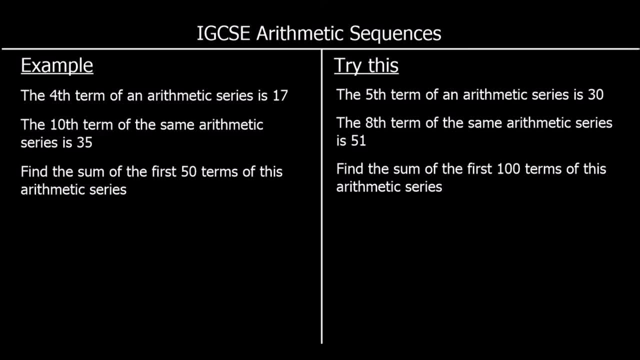 So that's the hours in the first five terms. And so what we need to do is consider a number. 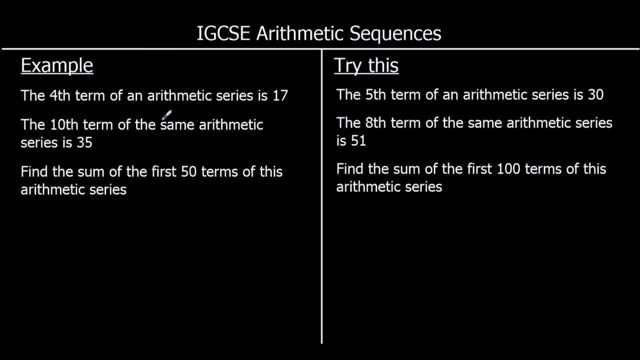 Try and guess what that means. It's not something we can compute in the formula, which we thought what does come in and where there is a value. Harmony in the equation. So yes. 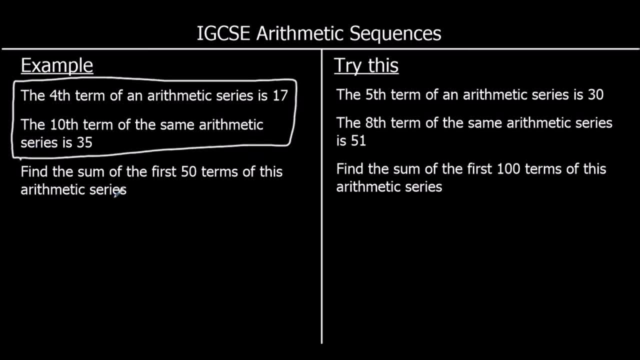 And once we know what a and d are, we can substitute in to the sum formula. 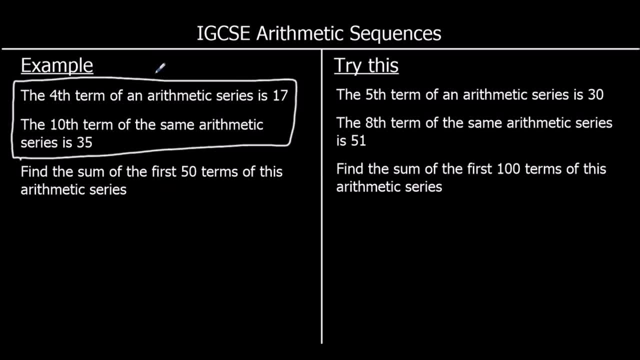 So the fourth term, well to find that, we're going to use our nth term formula. So un, the nth term, is a plus n minus 1 times d. 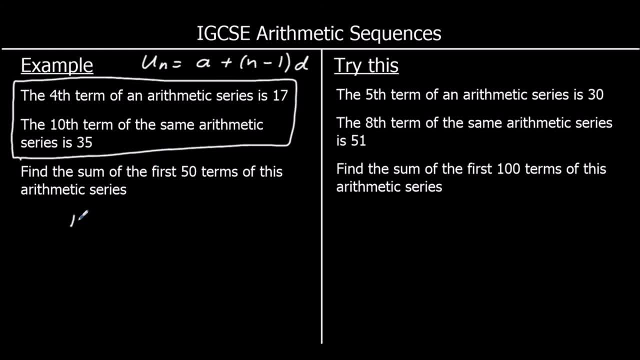 So the fourth term is 17. So 17 is a plus 4 minus 1, which is 3 lots of the common difference. 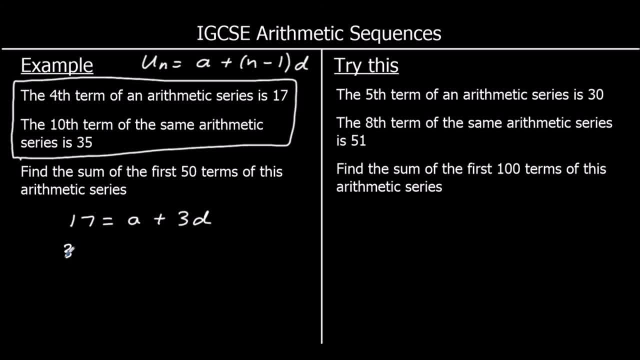 And the 10th term is 35. So 35 is the first term plus 10 minus 1, 9 lots of the common difference. 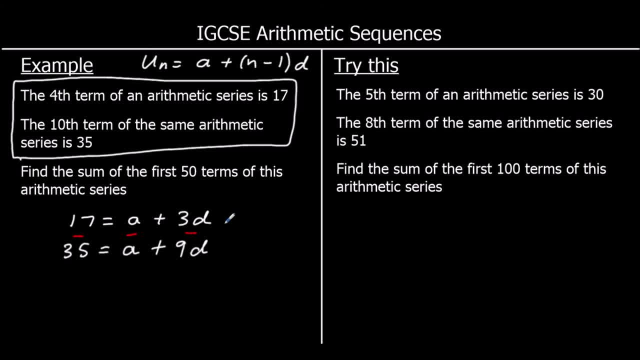 So to solve these simultaneous equations, well, we're going to take the top one away from the bottom one again. So 35 take away 17 will give us 18. 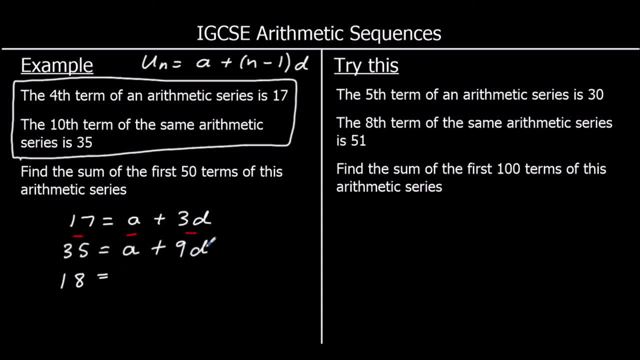 a take away a is nothing. 9 d's take away 3 d's is 6 d's. 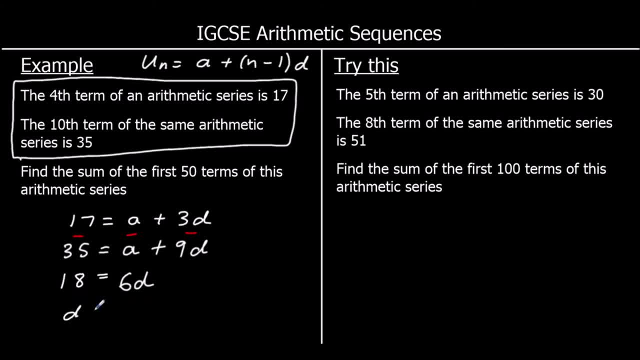 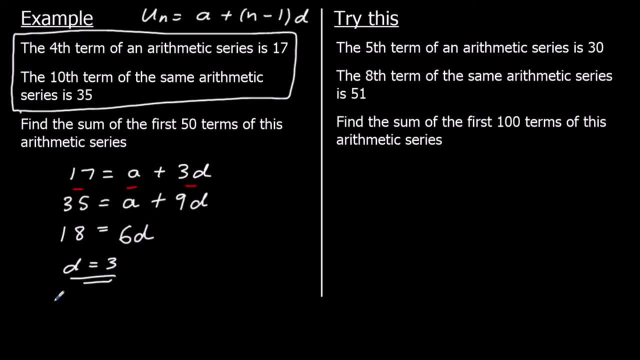 So dividing both sides by 6, we've got the common difference of 3 again. Now we can find a by substituting in. So 17, substitute in to the top line here. Is a plus 3 lots of the common difference, which is 3. 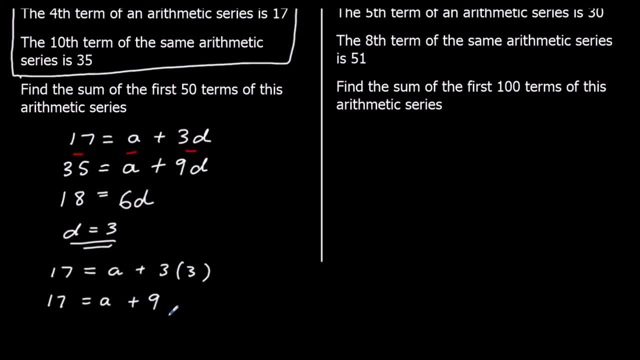 17 equals a plus 9. Take 9 away from both sides. So the first term is 8. 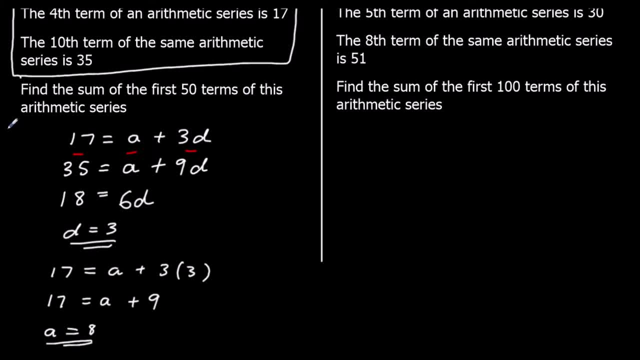 So now we can use the sum formula. We want 50 terms. So the sum of the first 50 terms. So n is 50. 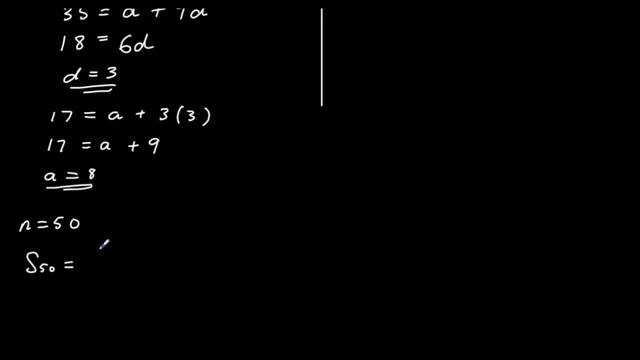 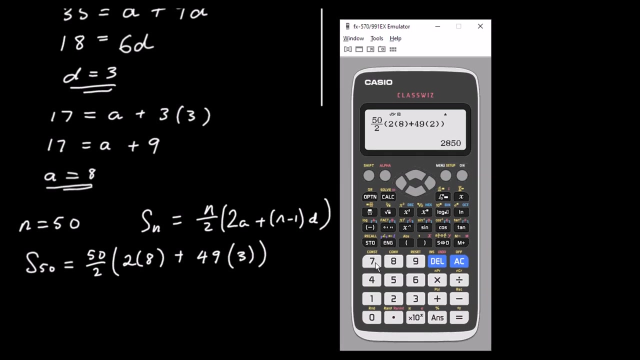 So the sum of the first 50 terms is n over 2. So the formula is Sn equals n over 2 times 2a plus n minus 1d. So 50 over 2 times 2a's, 2 8's plus n minus 1. 50 minus 1 is 49 times the common difference, which is 3. And again, we're going to type that into the calculator. So 50 over 2 times 2a, 2 8's plus n minus 1, which is 49 times the common difference, which is 3. And we've got 4075. 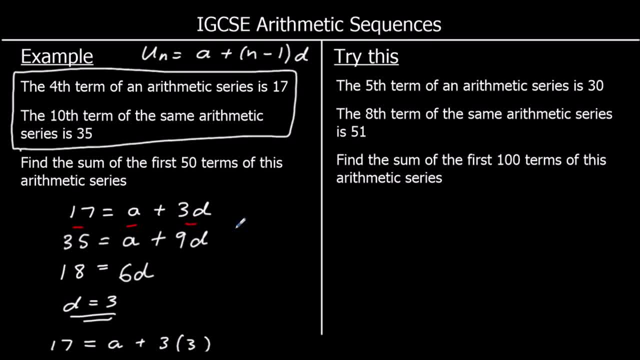 Okay, one for you to try. Okay, so pause the video. And give it a go. 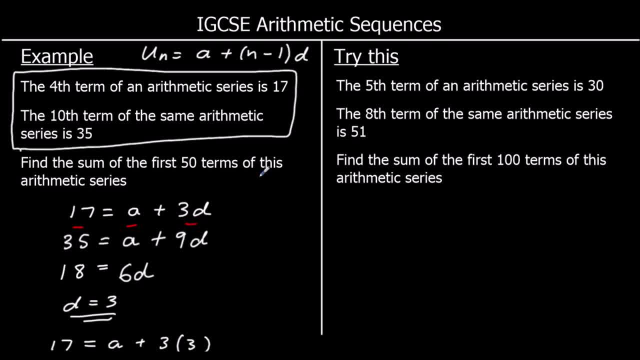 So we've been given the fifth term is 30. So 30 is a plus 4 lots of the common difference. The eighth term is 51. 51 is the first term plus 7 lots of the common difference. We're going to solve these simultaneous equations to find a and d. So bottom equation. 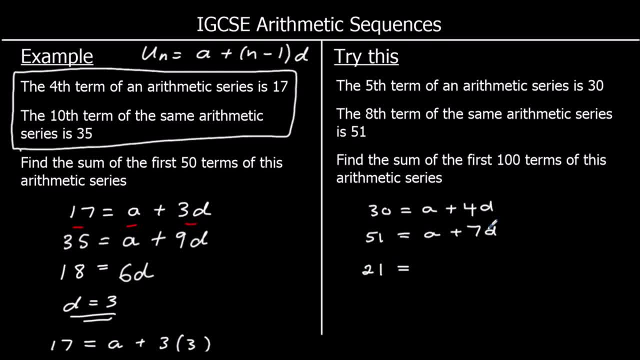 Take away top equation gives us 21 equals 3d. So dividing by 3, the common difference is 7. 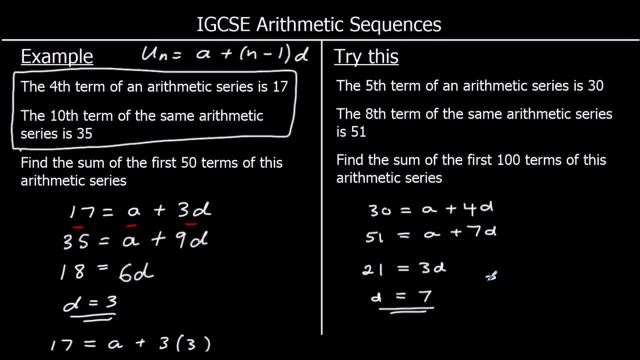 Substituting back in to the top equation, 30 equals a plus 4 7s. 4 7s are 28. 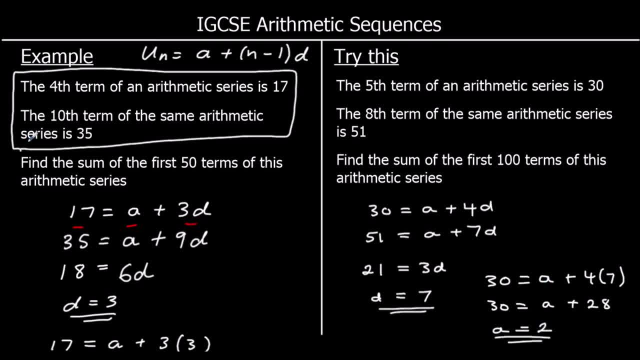 So take 28 away from both sides, we get a is 2. 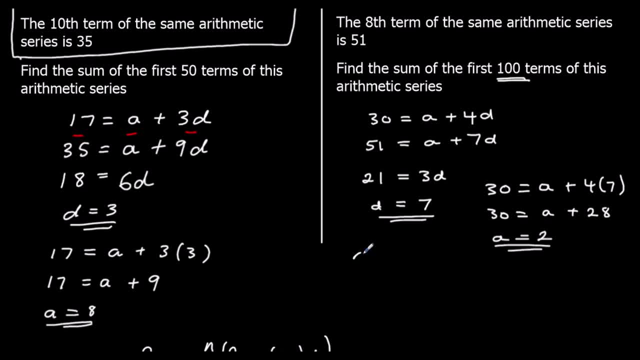 We want to sum of the first 100 terms. So n is a hundred. So the sum of the first 100 terms is. 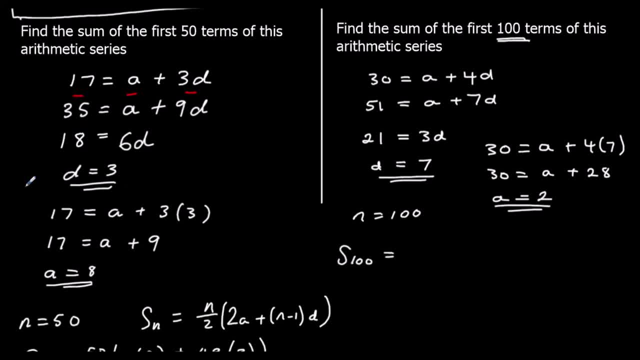 So using our SUM formula again, which is down here. 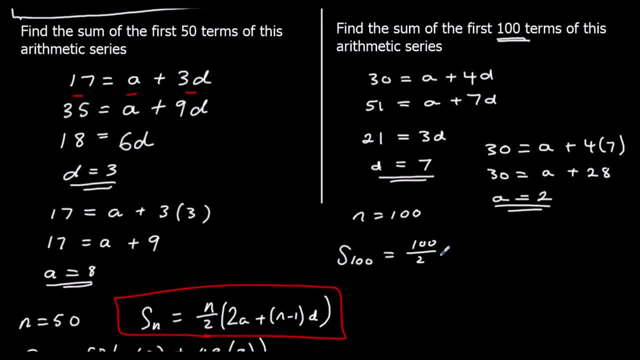 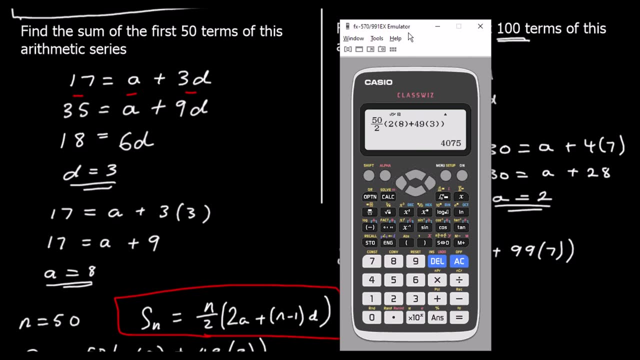 So 101 times two a's. Plus n minus one, which is 99, one which is 99 lots of the common difference and we'll type that into the calculator 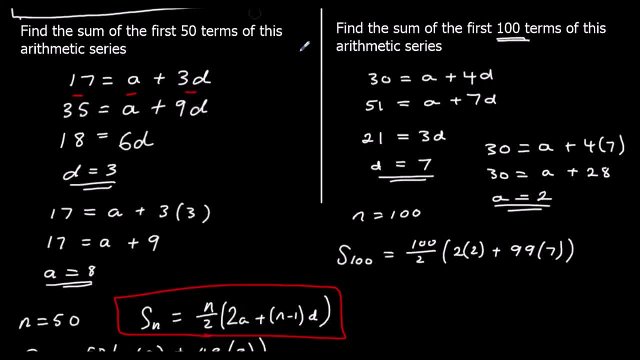 and we get out 34 850 and that's our sum of the first 100 terms